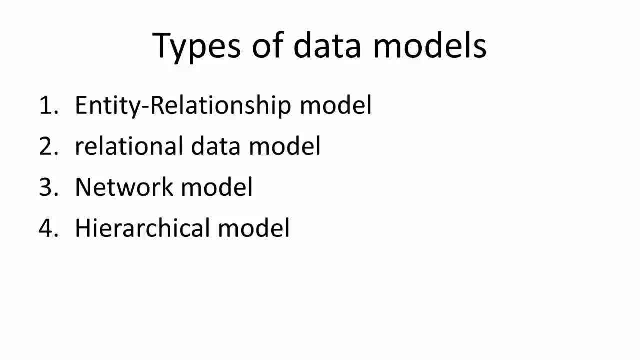 If the question comes: what are the types of data model? These are the four types of data model. I don't want you guys to get confused between types and categories, So here I am explaining it in detail. So let's look at each type of data model and in which category they fall. 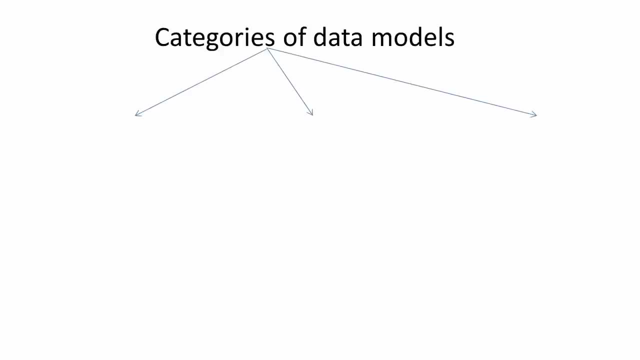 All right. So, as we have seen, we can look at this chart or this diagram. There are three categories: high level or conceptual data model, representation, representational or implementation data model and low level of physical data model. These are three categories. 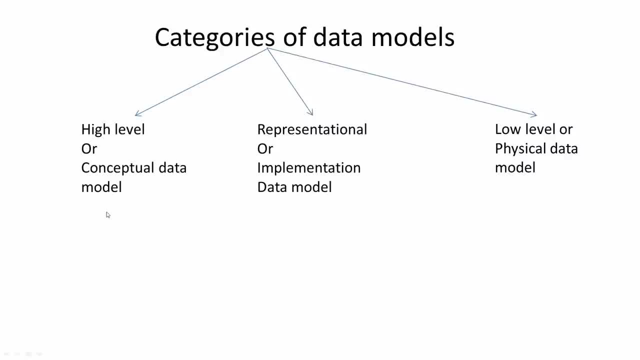 And in each category we have got different types of data. For example, high level data model. We have got an entity relationship model. It falls in the category of high level data model, All right. Then we have got representational or implementational category, in which we have got the three other data models. 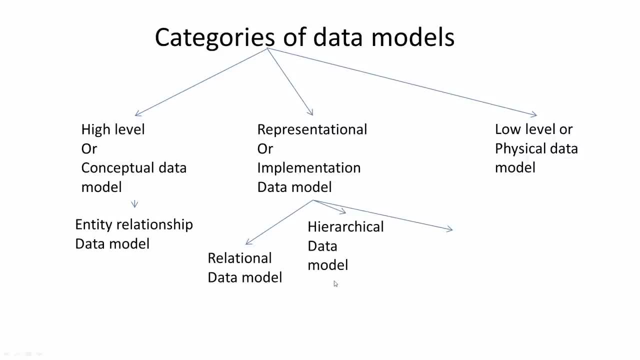 which are the relational data model, hierarchical data model and network data model. Now, if you want to know about low level of physical data model and what falls into that category, basically you just go and check the video on the categories of data model. 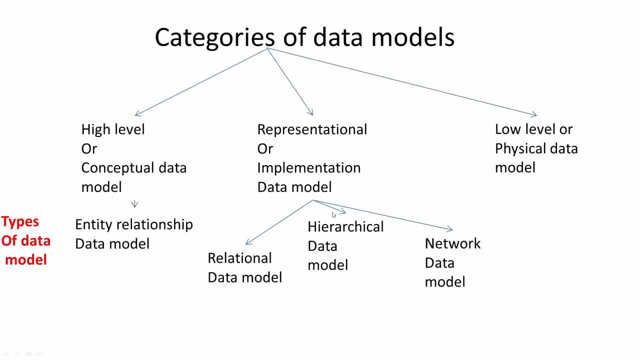 All right, So these are the main types of data model. There is no type of data model that falls specifically in physical data model. All right, So these are the four types of data model: entity relationship data model, relational data model, hierarchical data model and network data model. 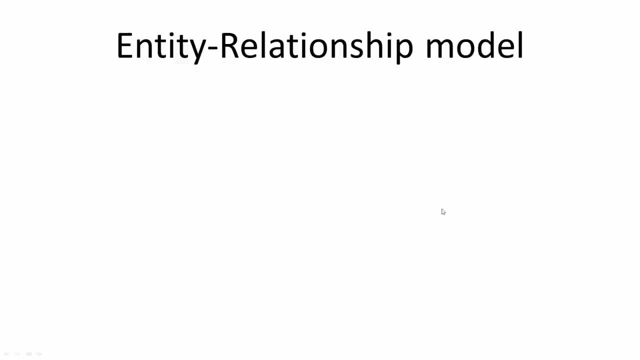 All right Now. first we look at entity relationship data model. What does that mean? As the name suggests, in this data model, what we have got is multiple entities that represent real world objects or concepts, such as an employee is an entity or a student is an entity. 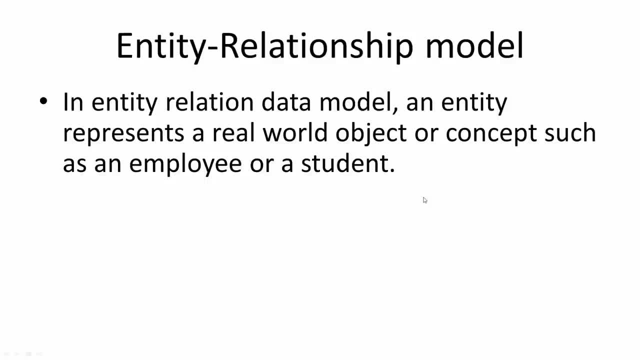 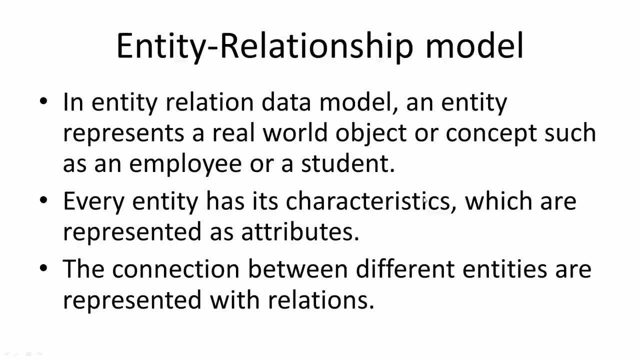 All right, So there are multiple entities in this data model and every entity has its own characteristics, All right, And these characteristics are called attributes in this data model. All right, Then we have got the connections between different entities. Now, just having entities doesn't make any use. 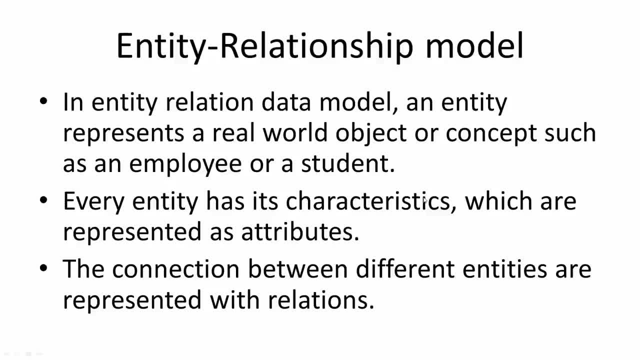 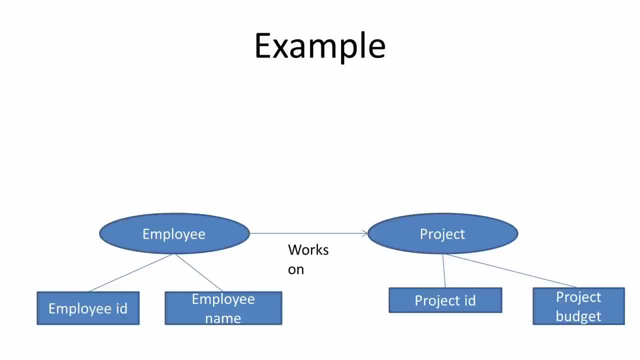 All right, So it doesn't make any sense. So hence we have to do the connection between these different entities to represent the data about them. All right, So this connection between different entities is represented as a relation, All right, So we look at an example so that you understand this concept much more easier. 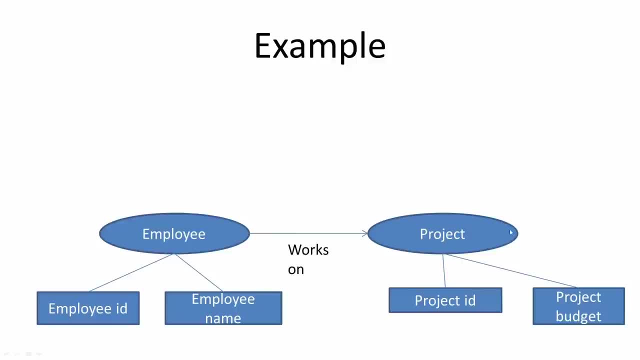 First thing, let's say we have got two entities over here, employee and project, All right, And, like we said, each entity will have its own attributes or its characteristics. So these attributes are: what for employee? employee ID, employee name? 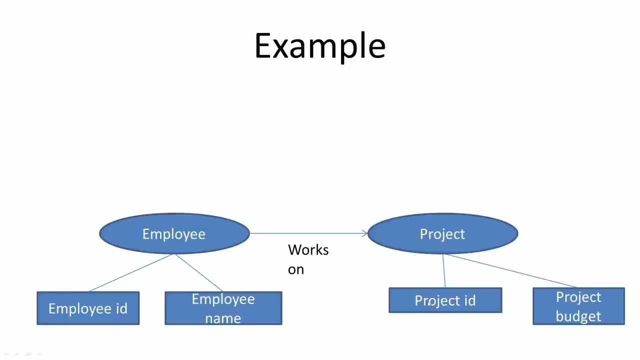 All right, And then we have attributes for the project. They're called project ID, project budget. Now, we have got the attributes, we have got the entities, But how do you connect them? Well, the employee works on a project, So what is the relationship between this employee and project that the employee works on? 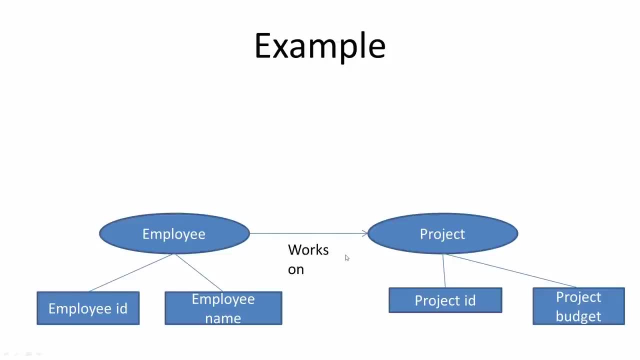 So works on, becomes the relationship between these two entities. So this is the basic of entity relationship model. All right, Now let's look at the next model, which is called relational data model. A relational data model uses the concepts of database as collection of tables. 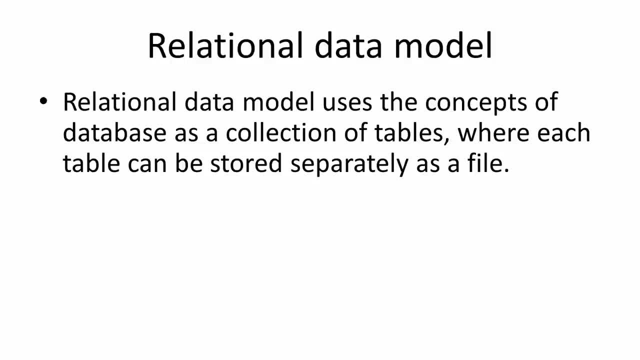 All right, Now in this table each, So in this database data model, each table is stored separately as a file, All right. And all the database operations are done with relations between the tables. Now, most relational database use high level language like SQL. 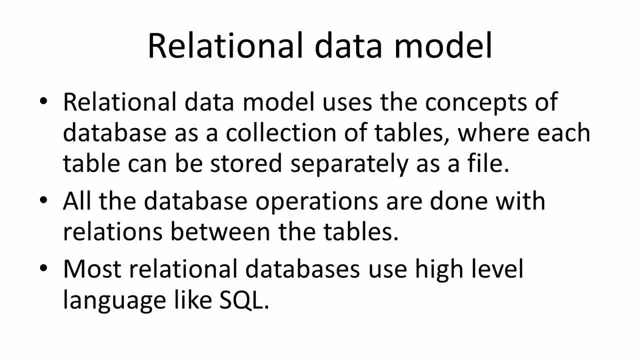 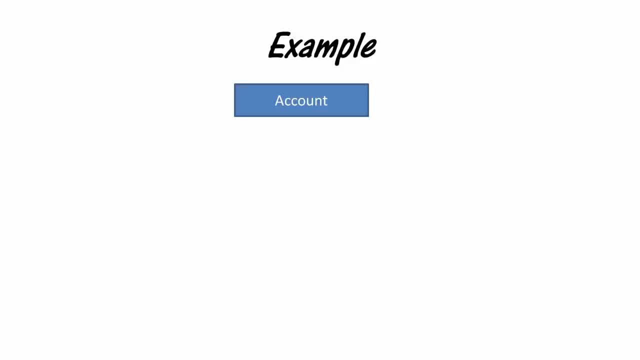 We'll look at an example so that you understand what do you mean by tables and what are the different components of relational data model. So let's say, for example, we have got a table called Or. we have got a relation called account. 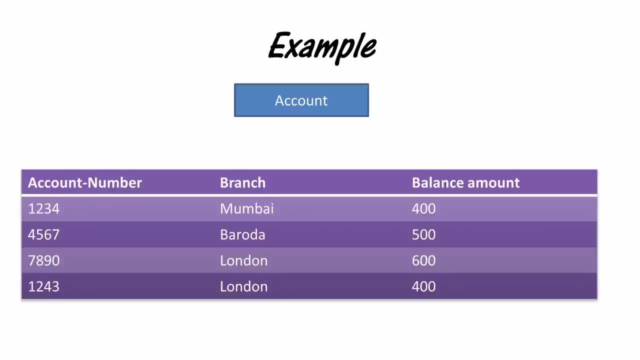 All right. Now this account Table. we have got three columns, All right. These columns are account number, branch and balance amount. So these three are the attributes of the entity account. All right, Don't get confused between entity relationship. 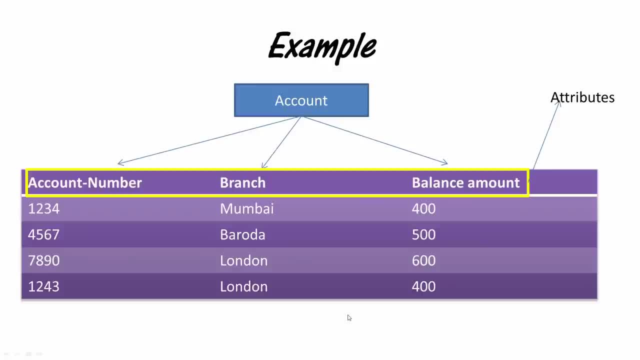 But I'm just telling you the terminology, like how you know from the last example. All right, So account number, branch and balance: account becomes the attributes of the account. All right, Now what about the row? Each row represents the information related to that row itself. 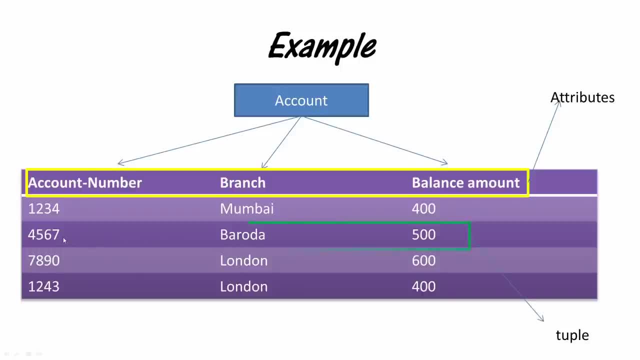 All right. So let's say we have got an account number here called four, five, six, seven. Now the account numbers related branch, that is the branch where the account number is, is Baroda and the balance amount of that account number is 500.. 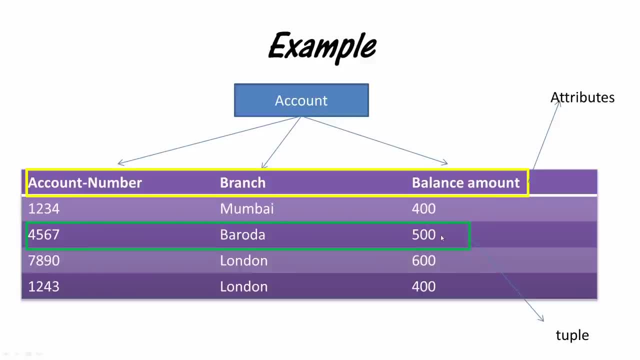 So all this information in one row is related to each other. So this row is called tuple in relational data model. Now you'll ask: what about the table? Sorry, what about the column? Now, as you can see over here, for example, branch. 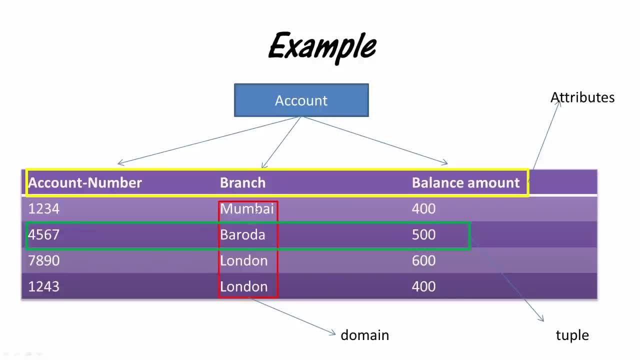 Now we have got branch Mumbai, Baroda, London, All right. So these are all called domain. You know why? Because this is a single type of information. Branch will contain only the type of information of one type, That is, it will have information about the branch. 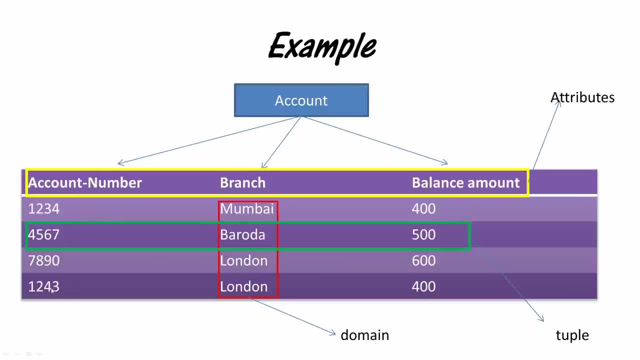 Account numbers will have only information in one type of numbers. All right, So it will be in that one data type only. Similarly, balance amount will be in integers, or let's say we'll have some decimals, but mostly it will be numerical value. 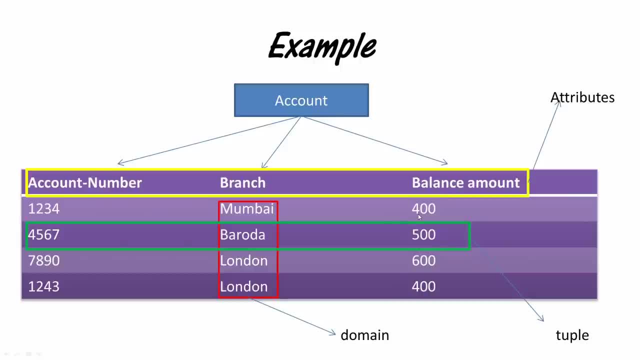 So it will be one type of information in one column, Hence it's called domain. So these are the different parts of relational data model. Now we'll look at an example how relational data model works. All right, So let's say we have got two tables over here. 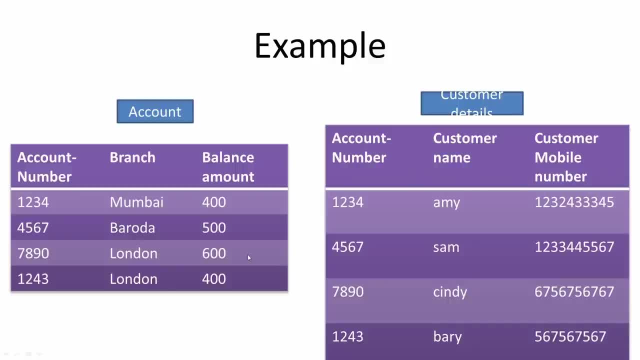 As I had told you, in relational data model you have the connections between the different tables to get the data or to do the processing on the database. Basically, let's say we have got two tables over here: One is account and the second one is called customer details. 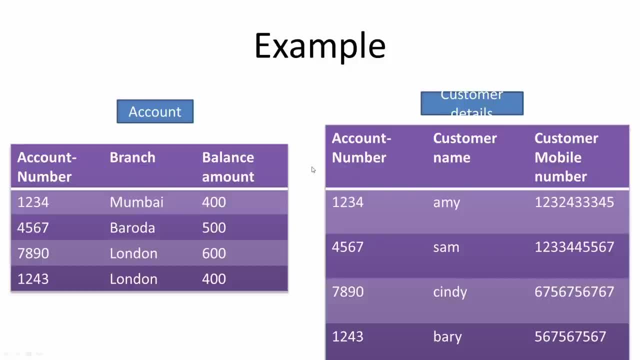 All right. So another thing you need to know is, in relational data model, a table is also called a relation, All right, So this is just a small detail that you need to know. All right, Now we have got two tables over here: account and customer details. 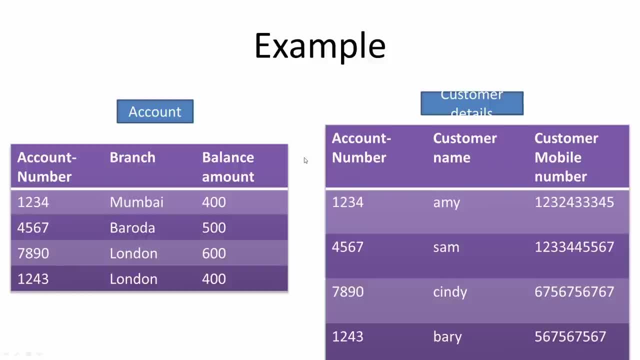 Now, how do we connect these two tables? Can you see something that is common in these two tables? All right, We have got the column account number, which is common in these two tables, All right. Now what this is called? It's called a key, basically. 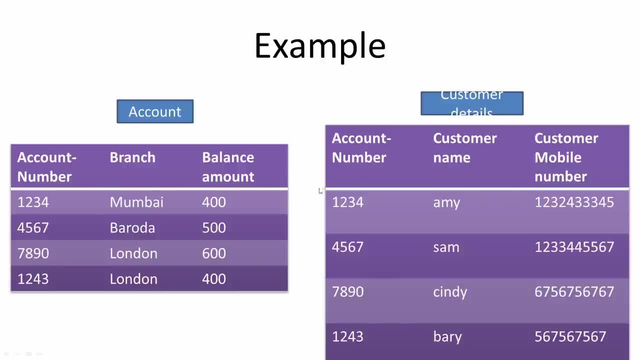 All right, If you want to learn about keys, I have a video on that. I'll put the link in the description. If you want to learn about the keys, you can go and check it out. All right, So I'll give you a hint or I'll give you the idea in general. 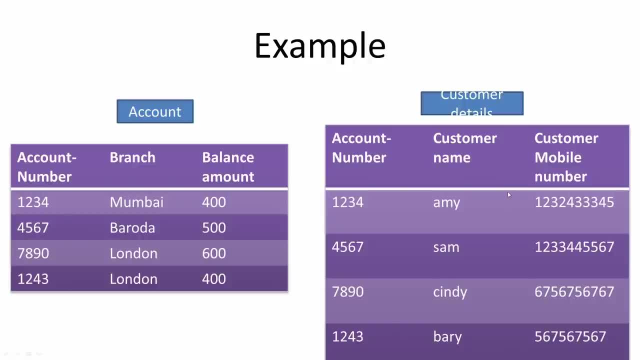 Basically, let's say you want to find out, let's say a customer wants to find out what is his current balance. All right, As we have seen, multiple banks have this option called miscall number, where you give a miscall and you find out what is the amount of balance that is there in your account. 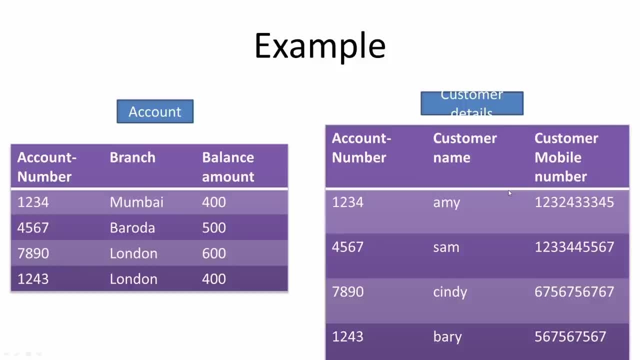 All right. So what that person does is that that person gives a call to the specific mobile number that the bank has provided. Now. the software receives a call from that number and it goes into the customer details to check which account number is associated with that mobile number. 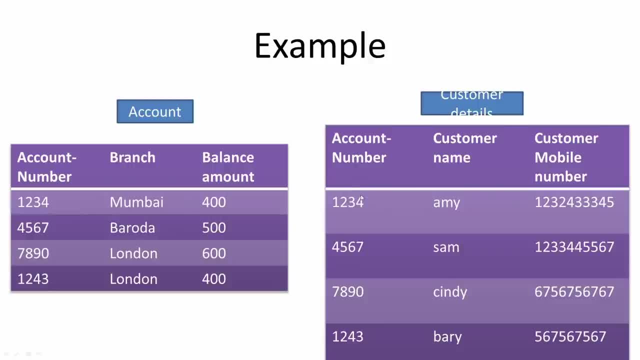 Now, once it gets the account number in the table, it will go and check that account number in the accounts table. All right, So it will be like, let's say, Amy is calling from her number, the system will get the call from this number and it will be like: OK, fine. 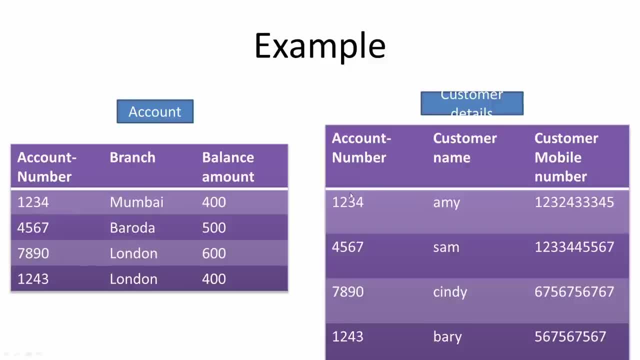 Just find out what is the account number associated with this mobile number And it will take that account number and it will go into the account table and it will be like: tell me what is the balance related to this account number. So one, two, three, four is the account number. 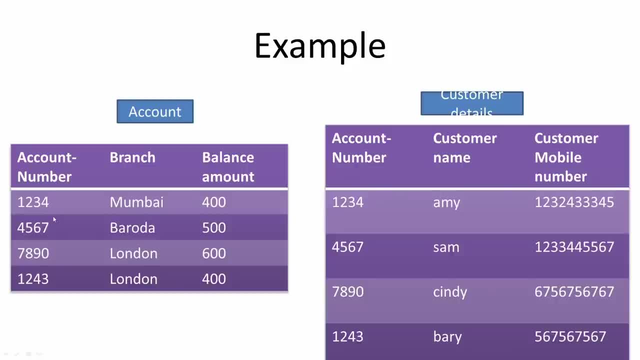 The balance amount is 400. The software is like: OK, now send an SMS saying that your balance is 400. So this is how you get information between tables and you connect the relationship Between them. All right, So this is how relational data model works. 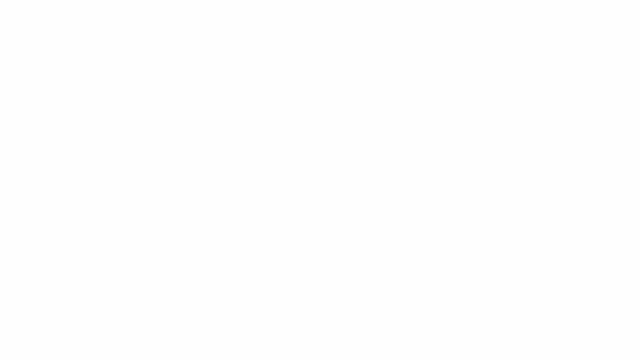 Now let's look at the next type of data model. It's called hierarchical data model. Now, this is a very simple data model. It is basically organizing the data in a tree like structure. All right, Let's say we have a company and that company has multiple departments. 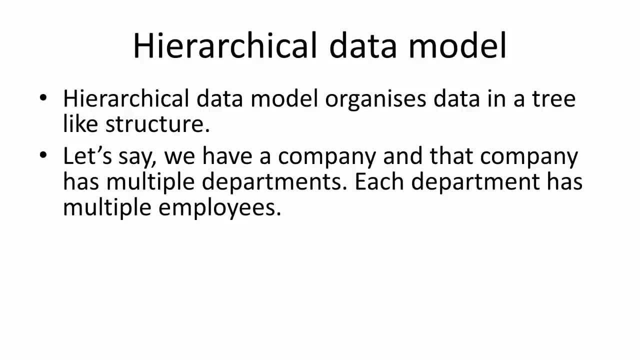 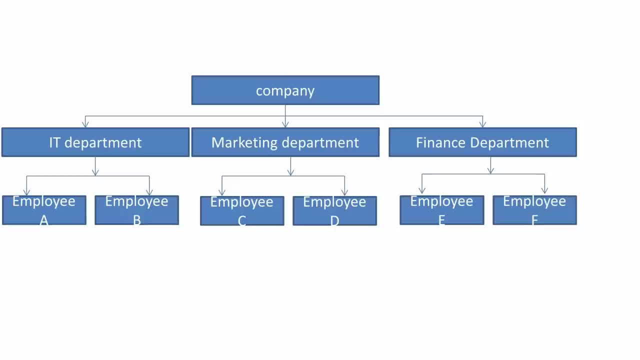 Each department has multiple employees, But one important factor of hierarchical data model is that each child node will have a single parent node. Remember this. It's like a tree. OK, so each child node will have only a single parent node. Let's look at an example. 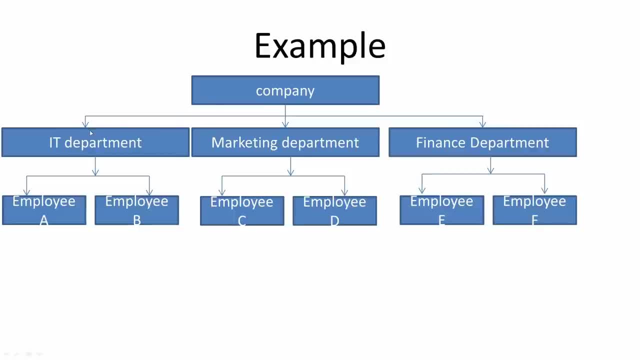 Let's say we have a company over here, All right. And in this company we have got multiple departments: IT department, marketing department and finance department. All right. Now each department has two employees. Let's say, IT department has employee A. 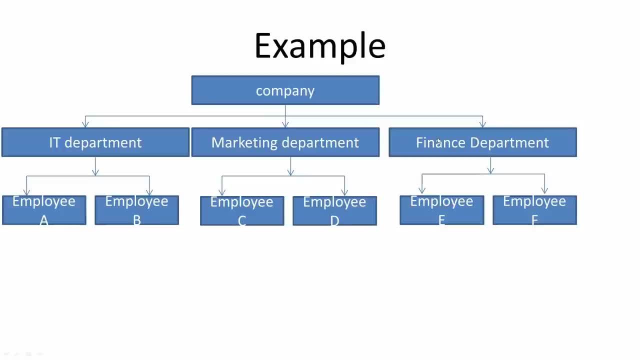 employee B, marketing department has employee C, employee D and financial department has employee E and employee F. Now employee A cannot work in IT department and marketing department at the same time. Neither can marketing department fellow work in IT or finance department at the same time.